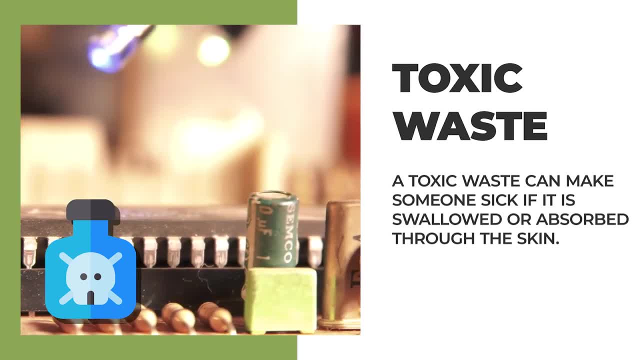 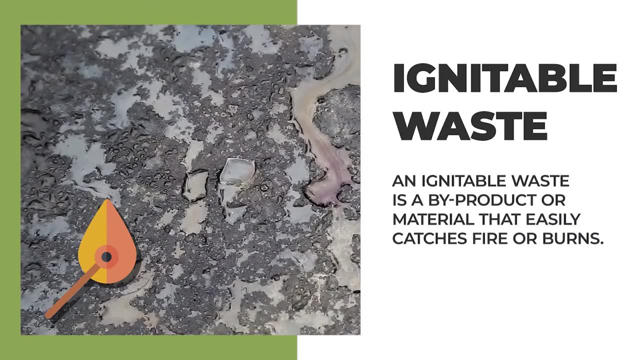 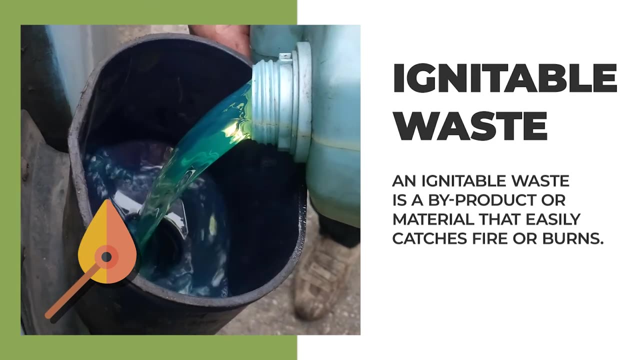 include fluorescent light bulbs. fluorescent light bulbs and fluorescent light bulbs. They contain mercury, and electronics like cell phones and computers that contain toxic metals like lead and cadmium. Another characteristic is ignitable wastes or materials that can easily catch on fire and burn. Gasolines and paint thinners are easy examples of this. 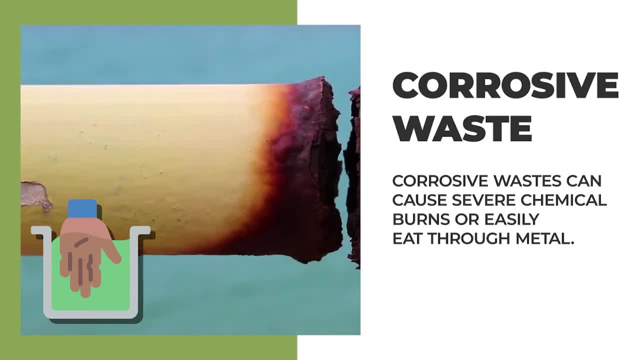 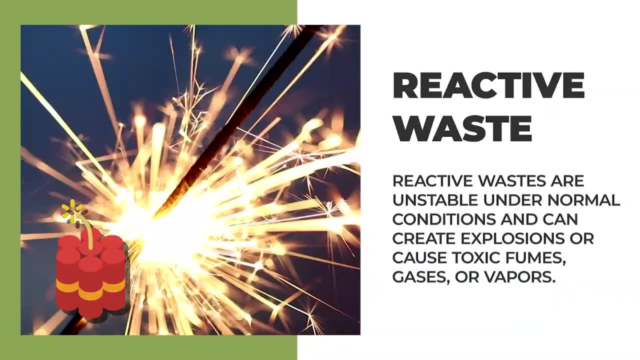 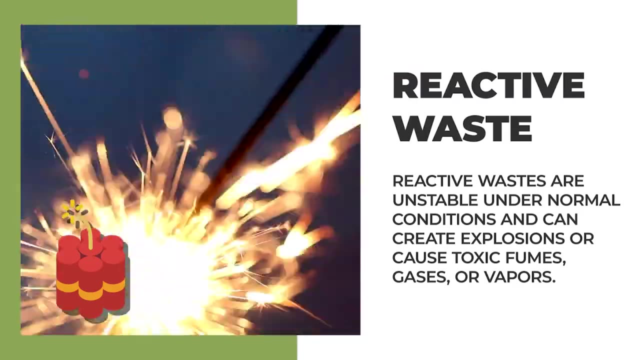 Next, corrosive wastes can cause severe chemical burns or easily eat through metal. Certain strong cleansers and acids can do this. Lastly, reactive wastes can be unstable under normal toxic conditions. When compressed, heated or mixed with water, they can cause an explosion. 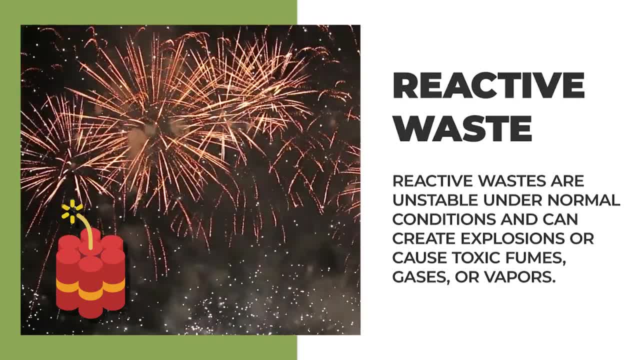 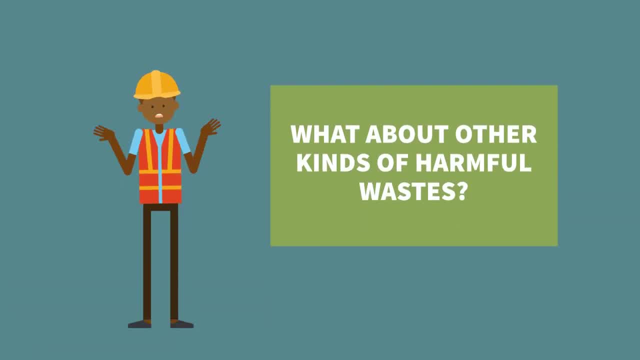 toxic fumes, gases or vapors. Examples of this are gunpowder and fireworks. You might have noticed that the definition of hazardous waste does not include every kind of waste that might be harmful: Radioactive materials, medical waste and solid waste. 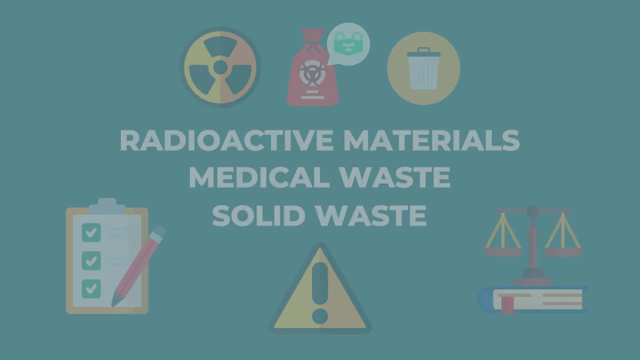 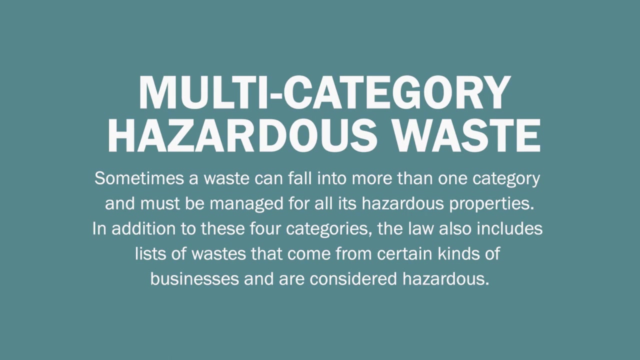 are dealt with under different laws than hazardous waste. Sometimes a waste can fall into more than one category and must be managed for all its hazardous properties. In addition to these four categories, the law also includes lists of wastes that come from certain kinds of businesses and are considered hazardous. 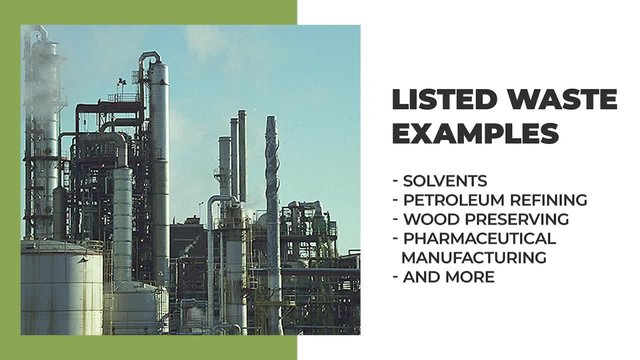 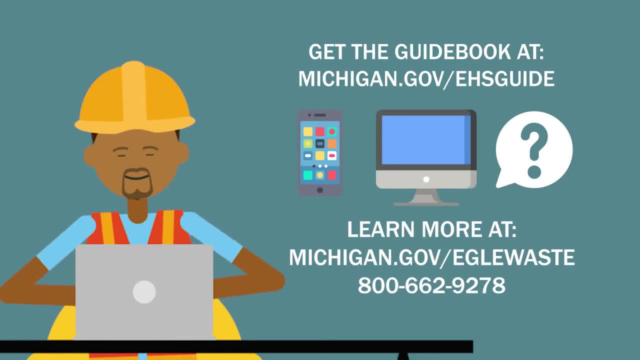 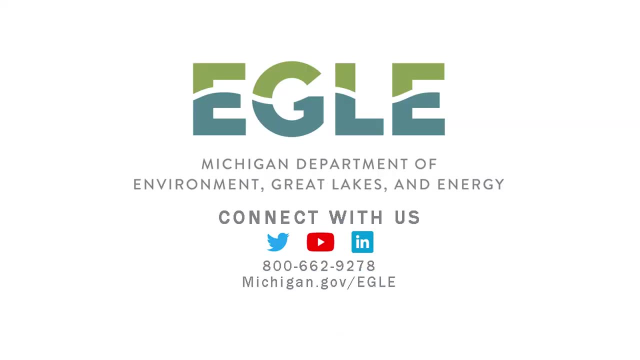 These lists include solvents, wastes from petroleum, refining, wood, preserving, pharmaceutical manufacturing and more. To learn more about hazardous waste regulations, check out our resources or contact our Environmental Assistance Center for help. Thanks for watching http//wwwhamskeycom.